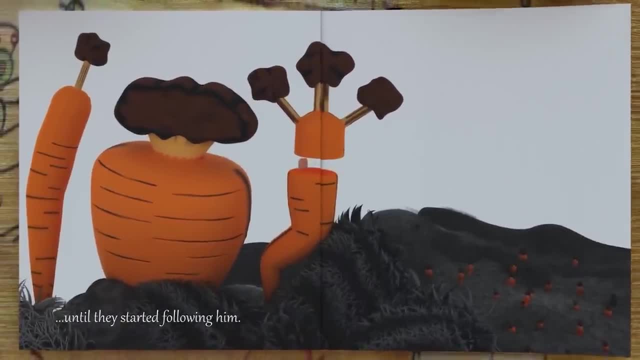 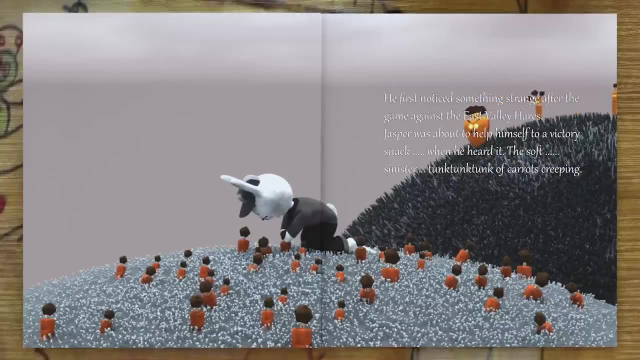 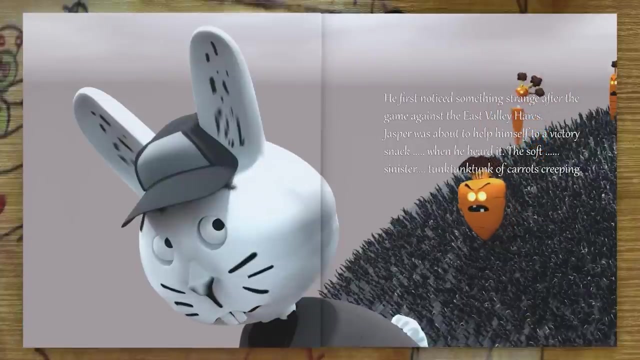 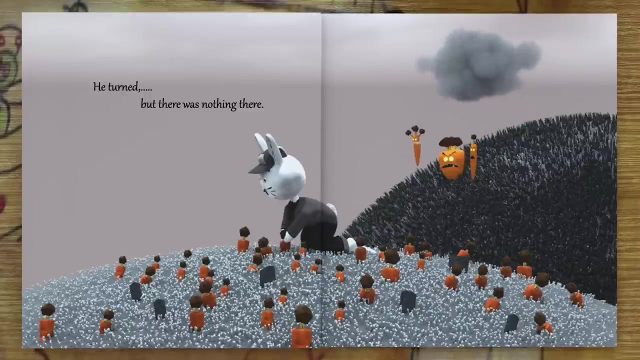 Until they started following him. That's creepy. He first noticed something strange after the big game against the East Valley. Jasper was about to help himself to a victory snack when he heard that the soft, sinister tonk, tonk, tonk of carrots creeping. He turned, but there was nothing there. 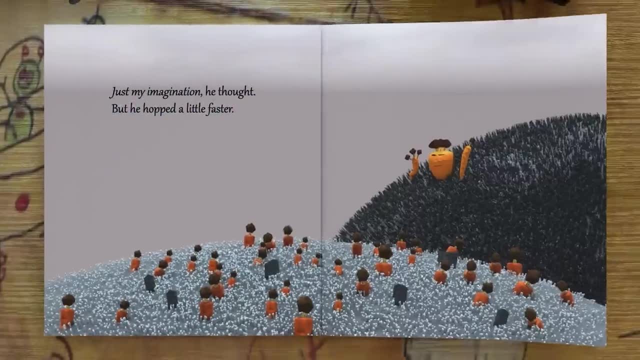 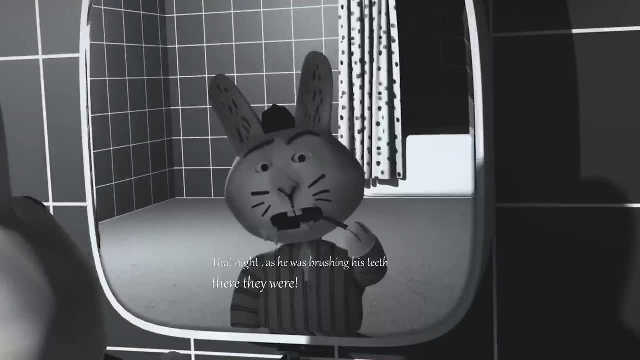 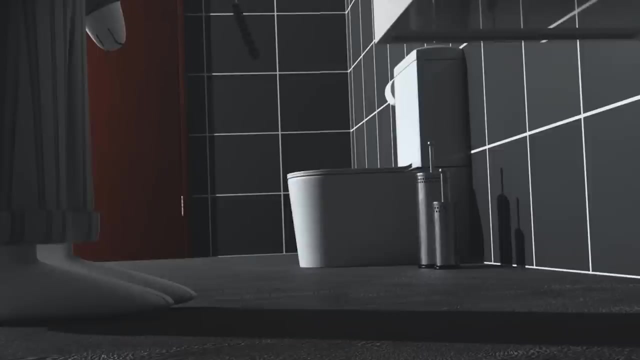 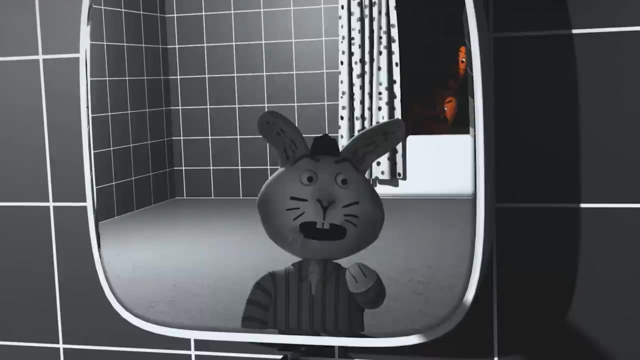 He thought, but he hopped a little faster. That night, as he was back to school, he heard the sound of the carrots creeping, Snapping the 不要, supposed to be a nice little snack. again He went out to the garden. 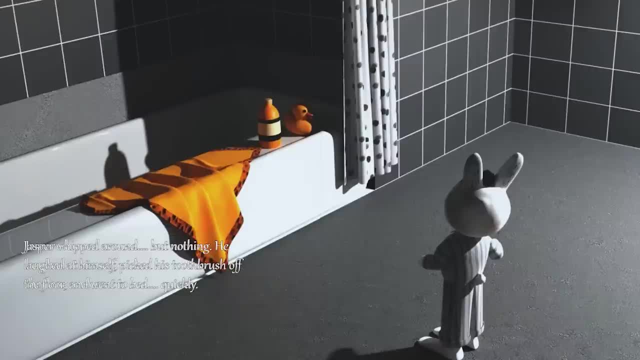 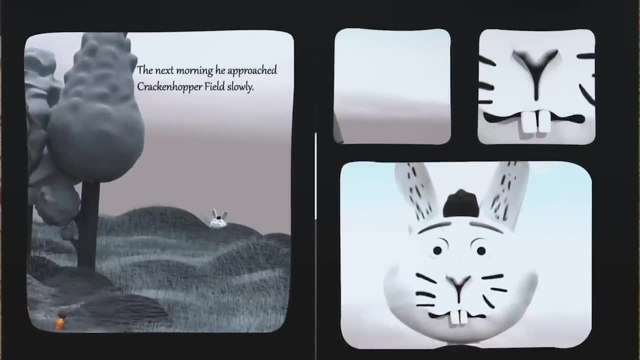 Williams was there. Apply it like a Gramps. He came back without pressure. He kept his teeth brushed. There they were Grass. He saiths the floor and went to bed quickly. The next morning he approached Kraken Hopperfield slowly. 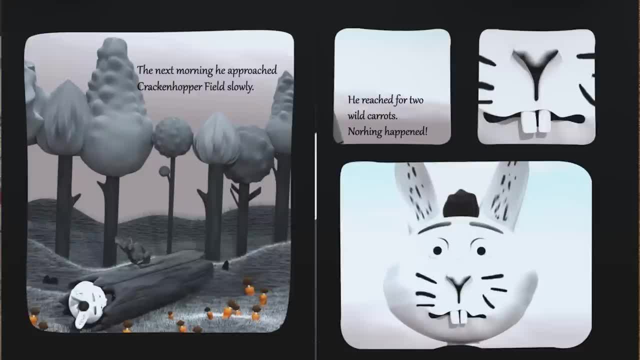 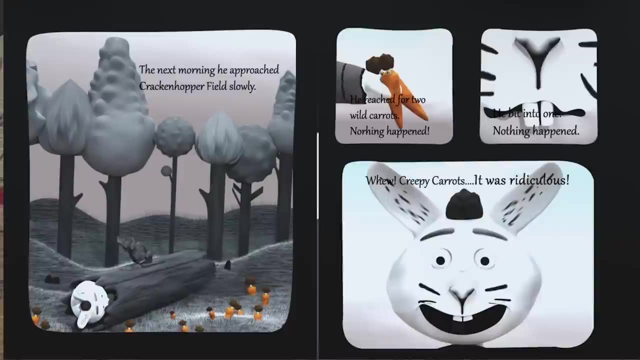 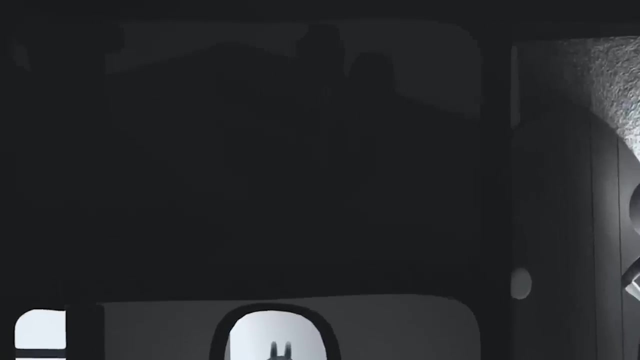 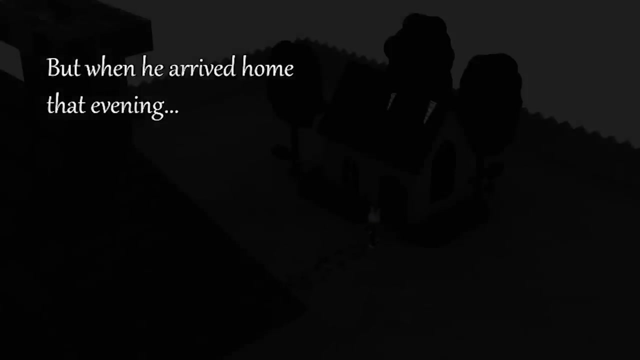 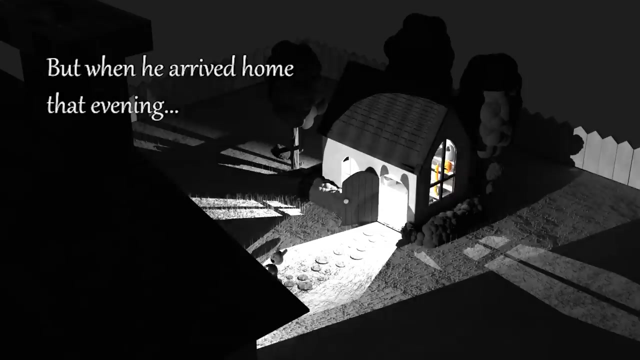 He reached for two wild carrots. Nothing happened. He bit into one- Nothing happened- Creepy carrots. It was ridiculous. But when he arrived home that evening something very spooky happened. Mom, Mom, Jasper screamed: Creepy carrots In the shed. 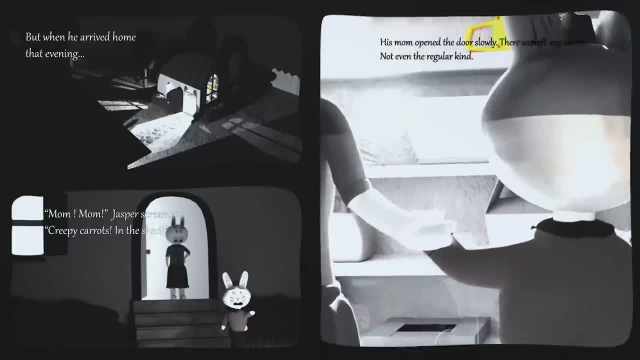 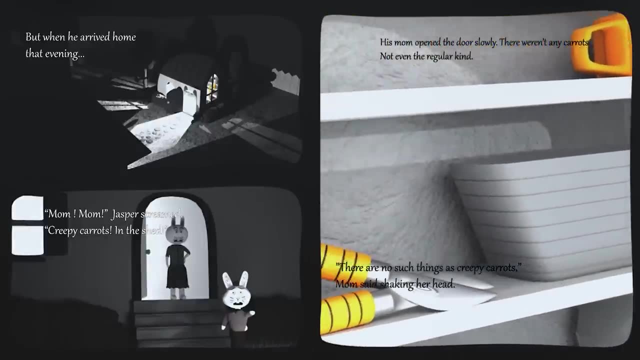 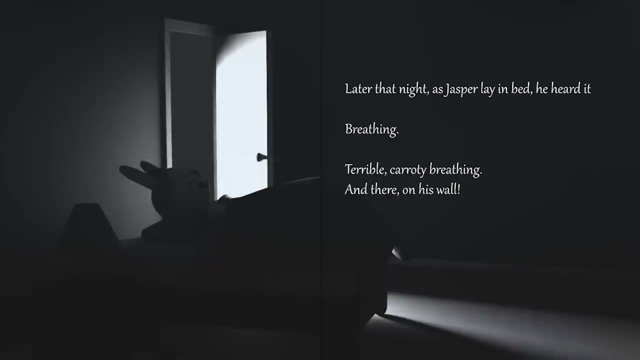 His mom opened the door slowly. There weren't any carrots, Not even the regular kind. There are no such things as creepy carrots, mom said, shaking her head. Later that night, as Jasper lay in bed, he heard it Breathing: Terrible carrot-y breathing. 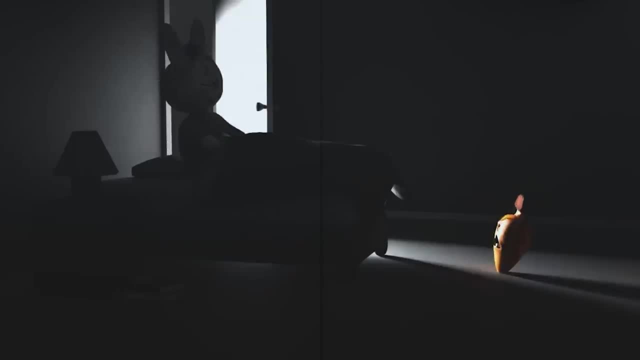 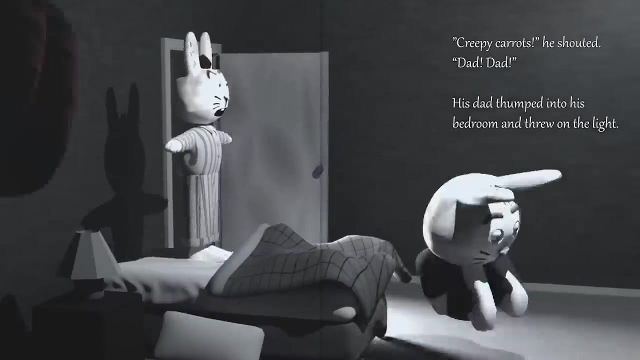 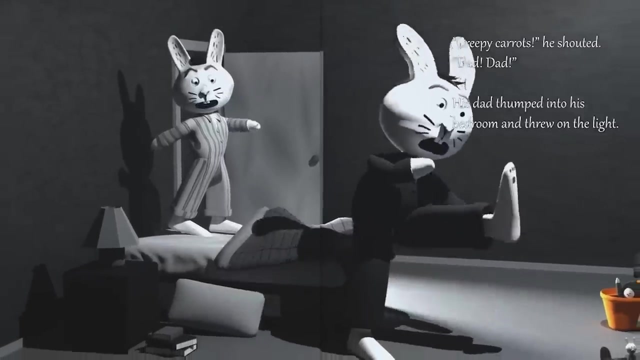 And there on his wall, Creepy carrots. He shouted: Shhh, Ahhh, Ahhh, Look, Look. His dad thumped into his bedroom and threw on the light. Where is it? Look Over there, Over there. 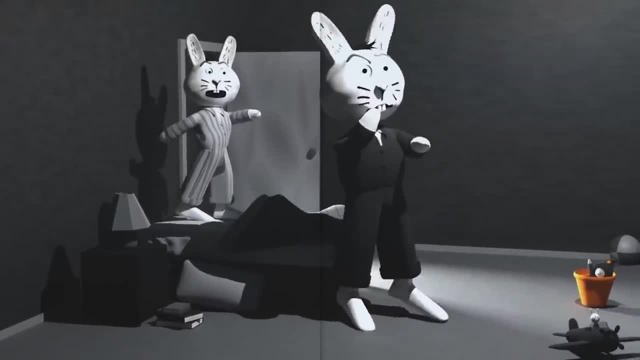 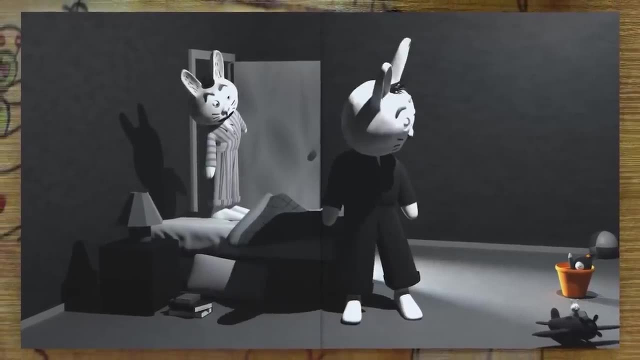 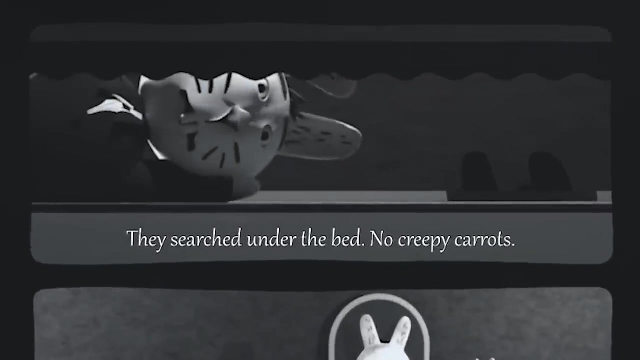 Look Daddy, Look Daddy, Look, Look Daddy. Look Where. Where That's not creepy carrots, No, It's all a dark scary. They searched under the bed. No creepy carrots, No Creepy carrots. 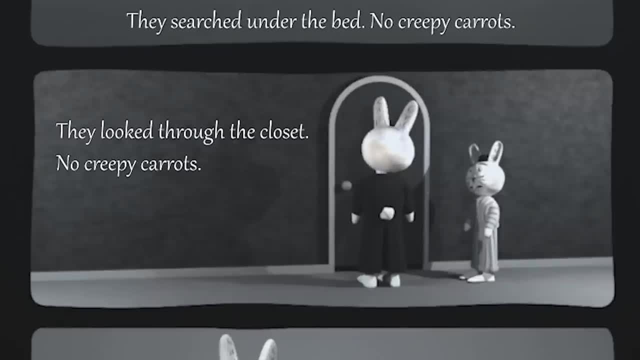 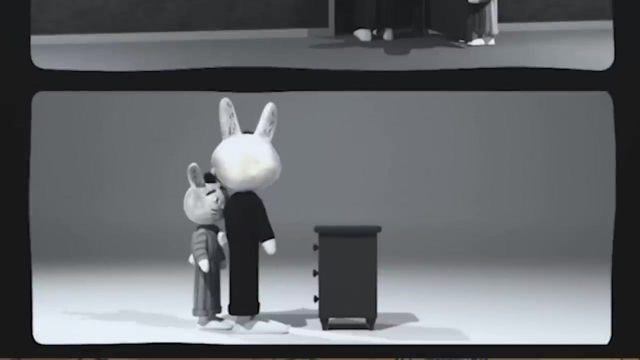 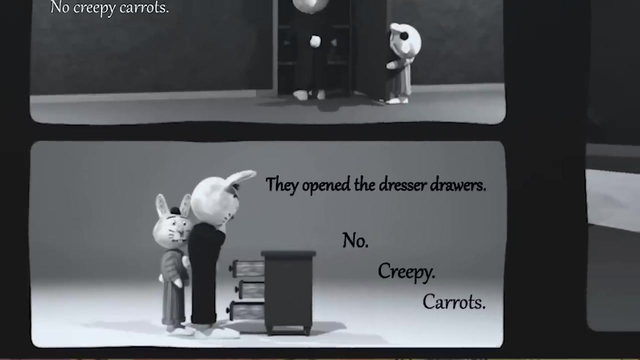 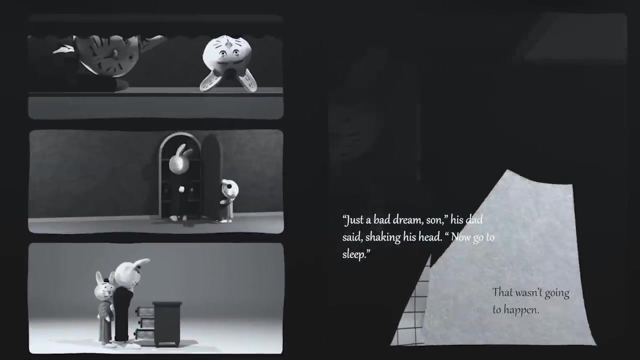 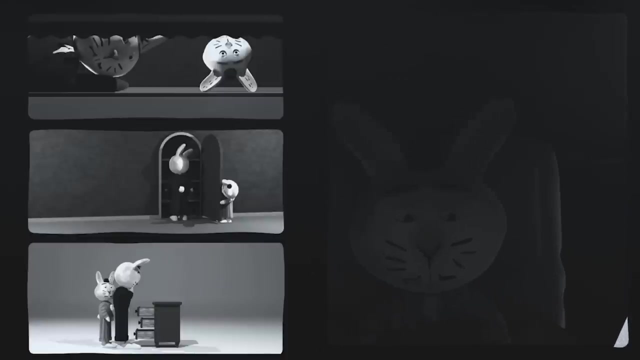 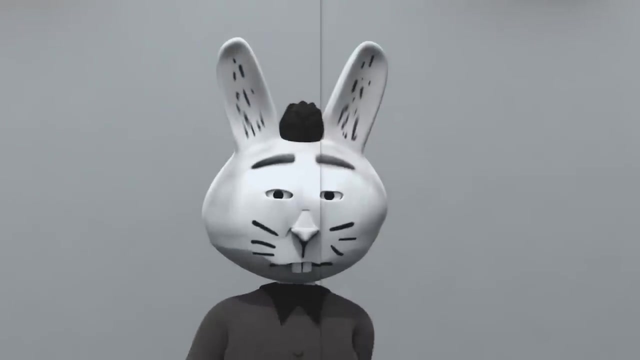 They looked through the closet- No creepy carrots. No Creepy carrots. They even opened the dresser drawers. No creepy carrots. Just a bad dream, son. his dad said, shaking his head: Now go to sleep. That wasn't going to happen. 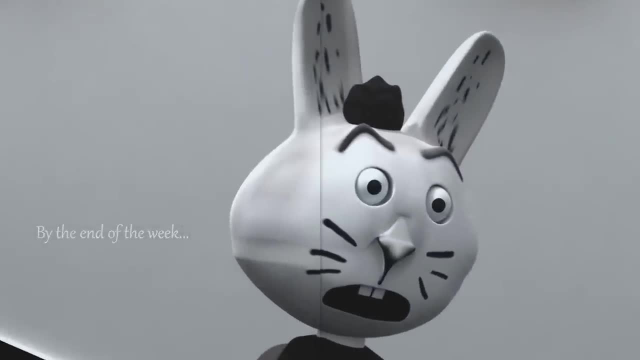 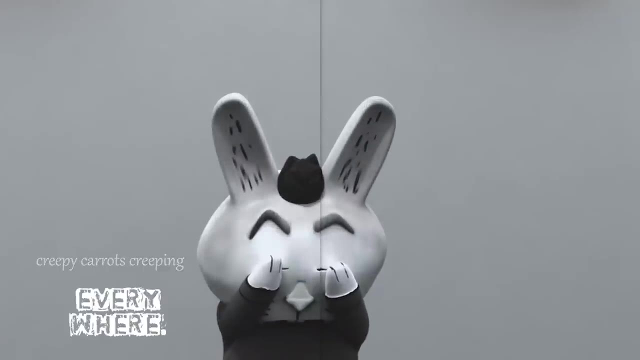 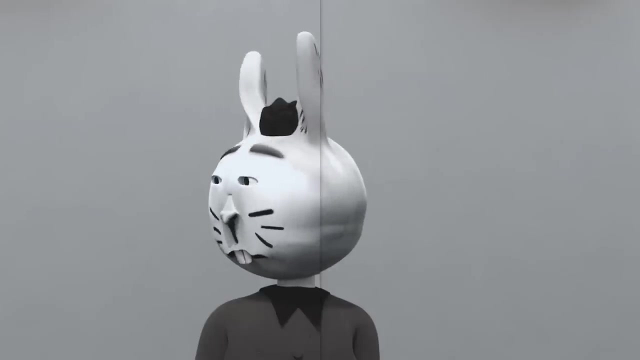 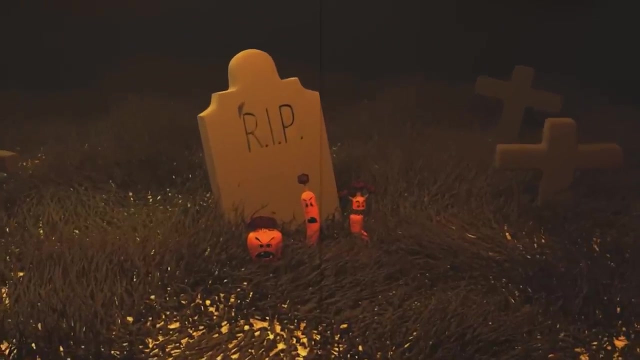 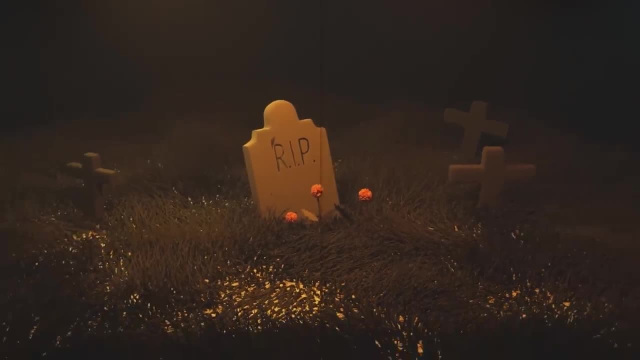 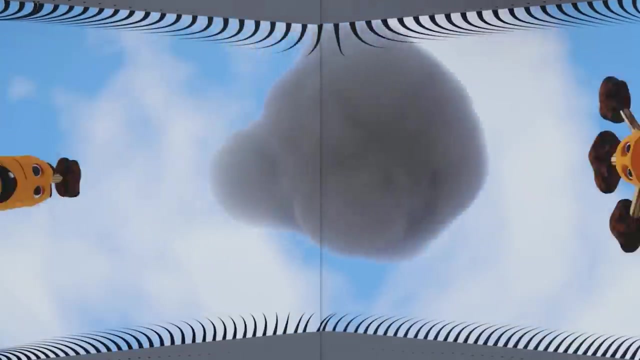 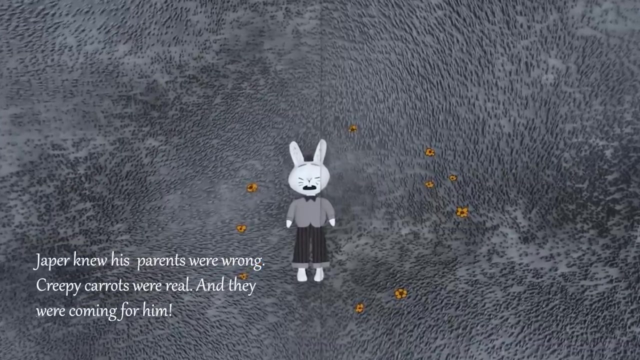 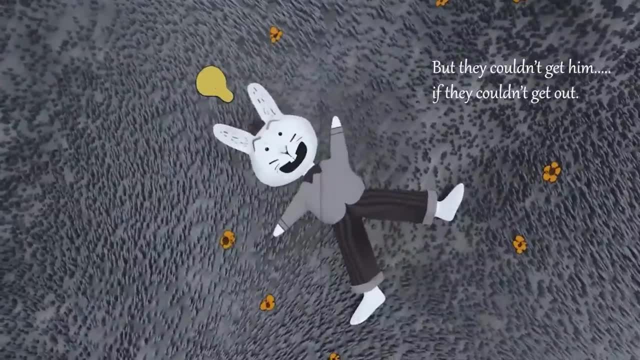 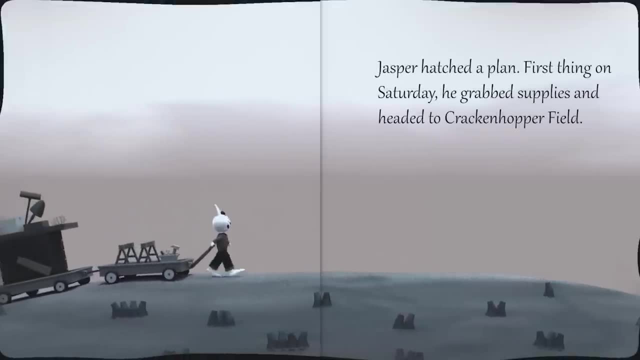 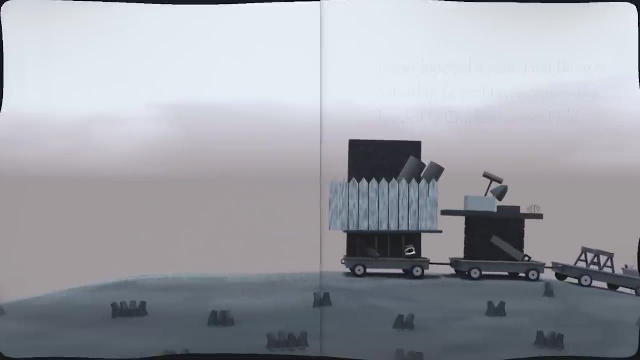 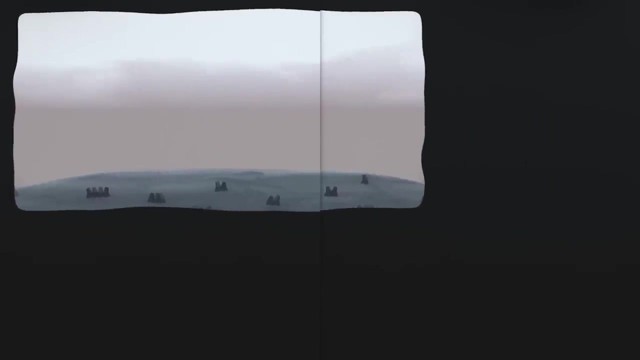 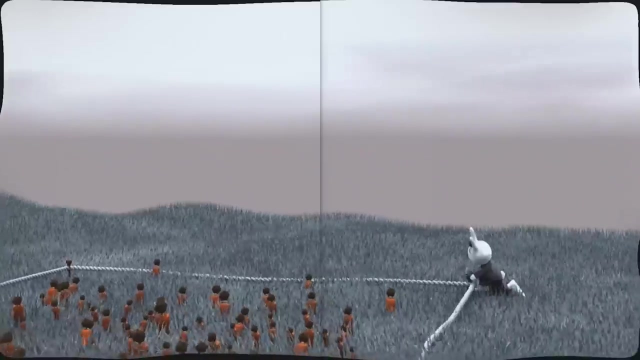 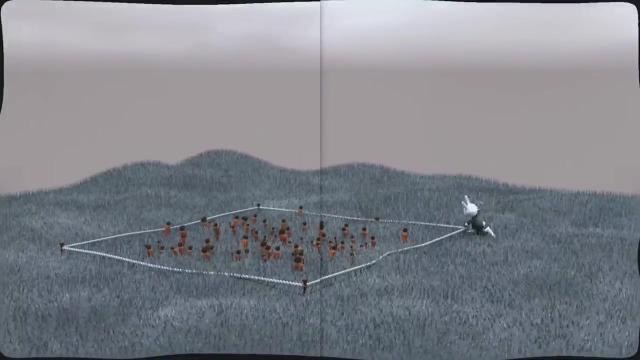 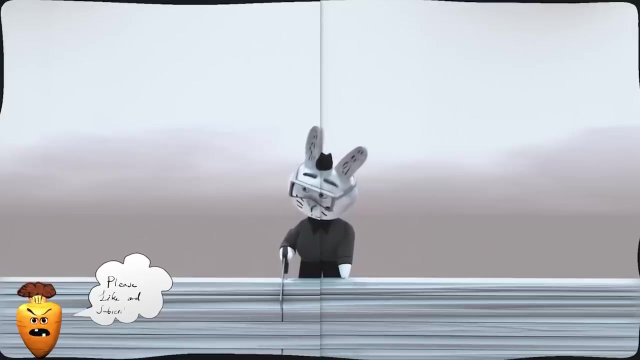 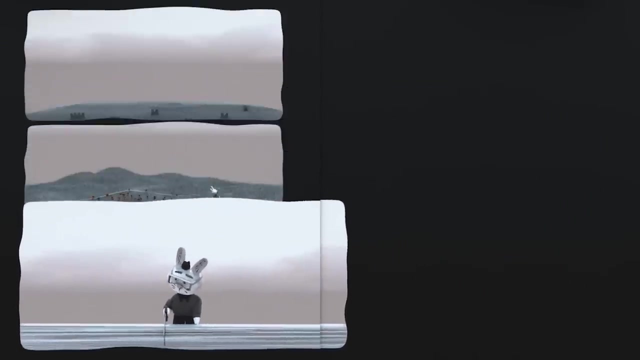 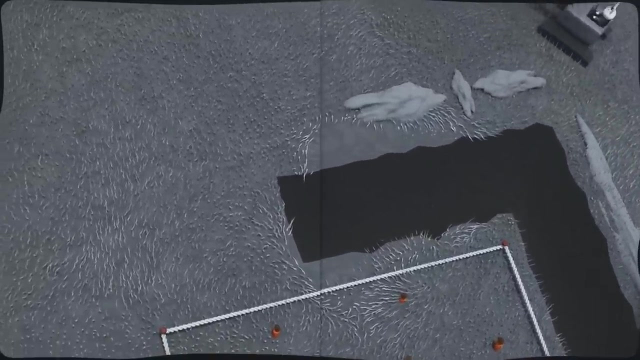 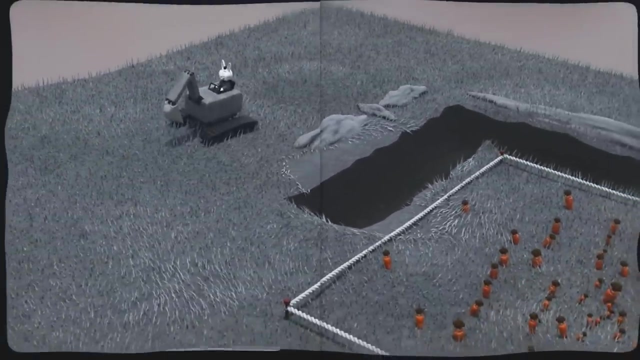 But they couldn't get him if they couldn't get out. Jasper then backed out. First thing on Saturday he grabbed supplies and headed to Krakenhopper Field. The next day he went back to Krakenhopper Field to get supplies and went back to Krakenhopper Field to get supplies and went back to Krakenhopper Field. 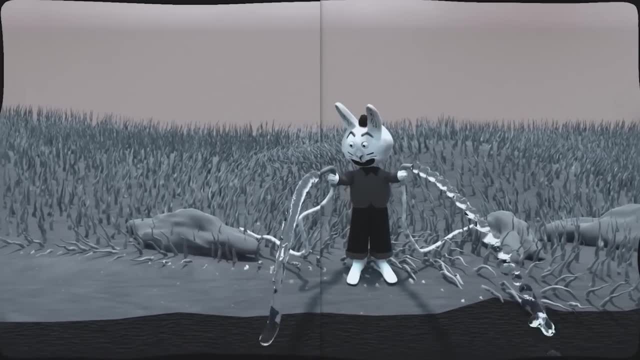 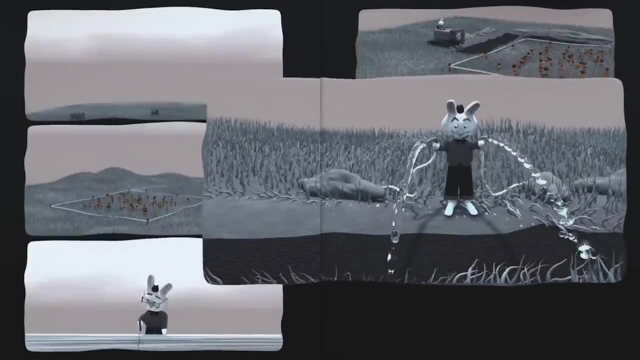 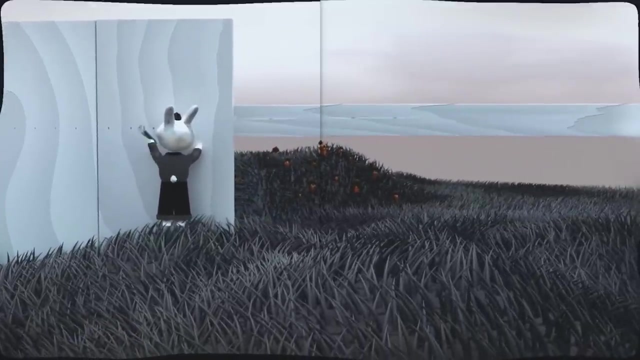 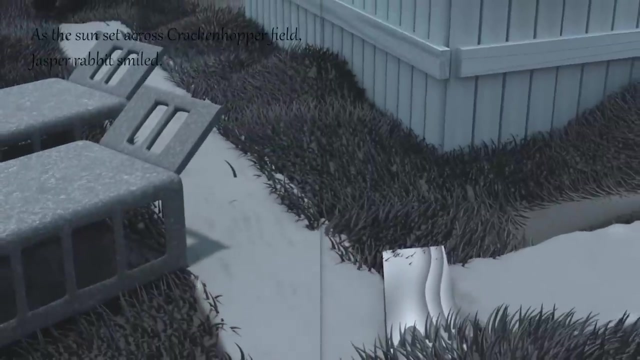 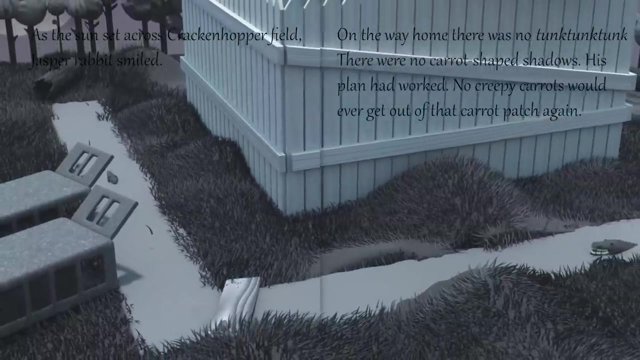 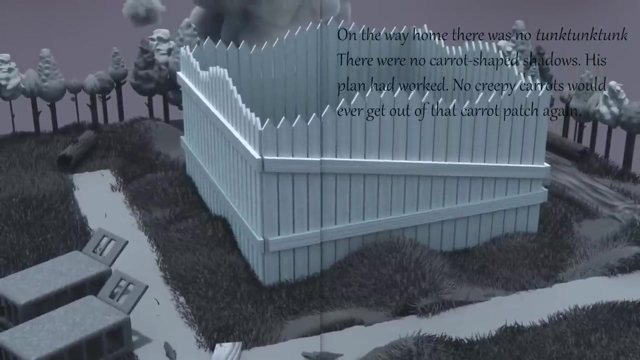 The next day he went back to Krakenhopper Field to get supplies and went back to Krakenhopper Field. There were no carrot-shaped shadows. His plan had worked. No creepy carrots would ever get out of that carrot patch again. 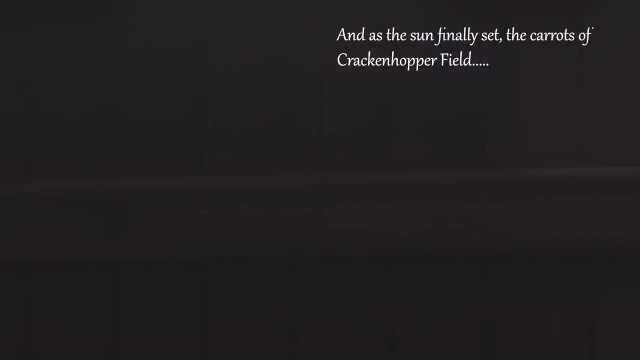 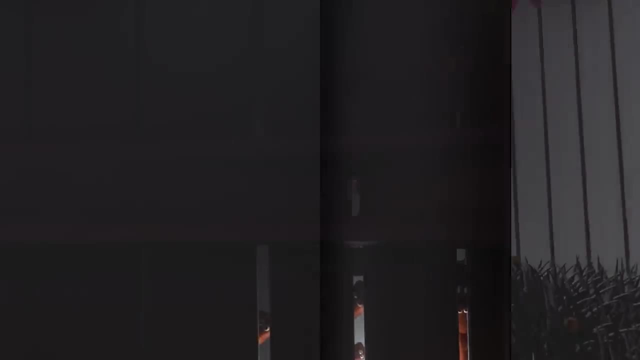 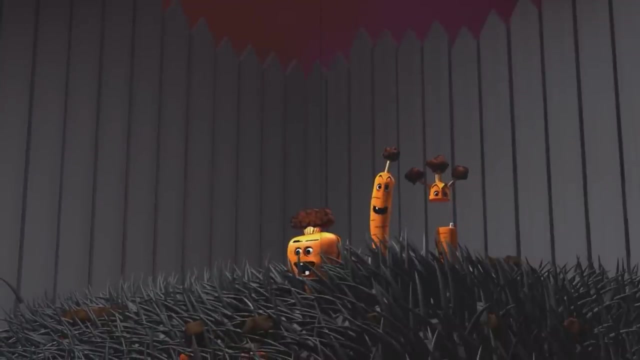 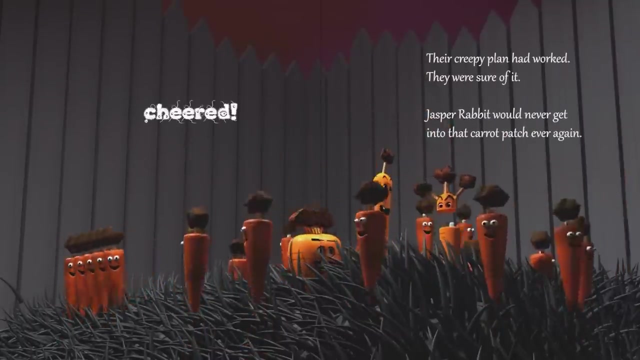 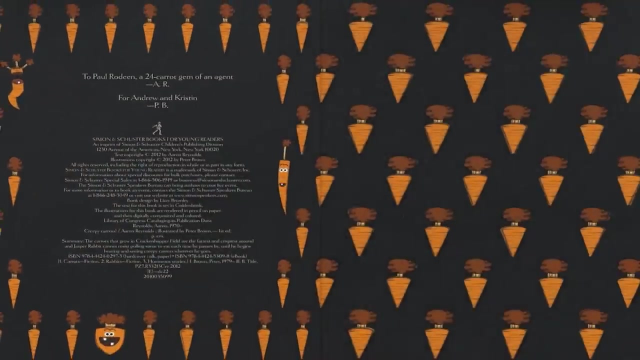 And as the sun finally set, the carrots were all gone. The carrots were all gone, The carrots of Krakenhopper Field Cheers. Their creepy plan had worked. They were sure of it. Jasper Rabbit would never get into that carrot patch ever again. 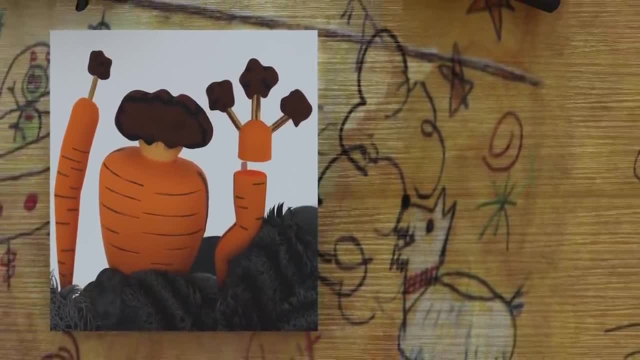 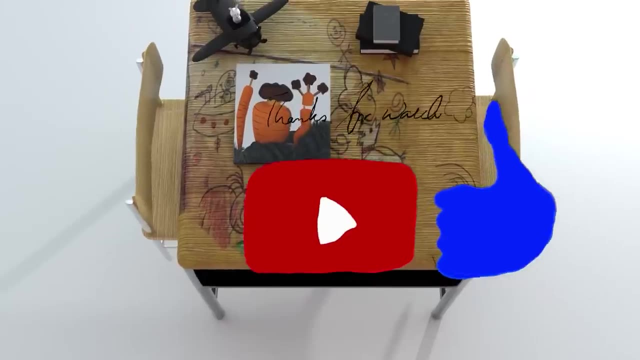 And that was the end of this story. And that was the end of this story. And that was the end of this story. Hope you enjoyed this beautiful story by Aaron Reynolds And animated by our channel- 5 Minutes with Uncle Ben. If you liked this story and also the animation, don't forget to drop likes. Till another animated storybook bye.